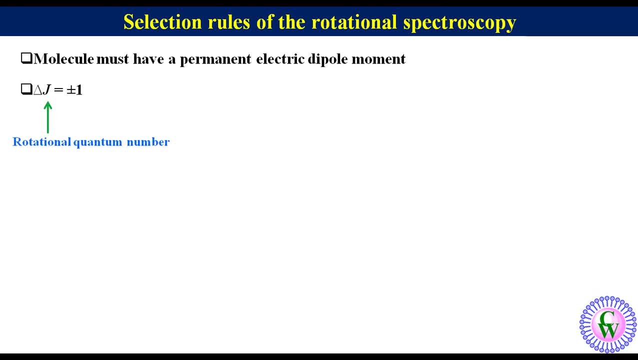 J is the rotational quantum number. that can be 0,, 1,, 2,, 3,, 4, etc. Let's understand first point with example. Suppose we have the list of these compounds in which we have to find which are rotationally active and which are inactive In the given. 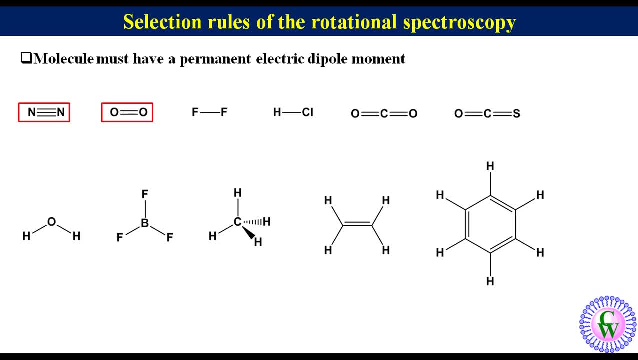 list of compounds: nitrogen oxygen, fluorine, carbon dioxide, boron trifluoride, methane, ethylene and benzene. In the given list of compounds: nitrogen oxygen, fluorine, carbon dioxide, boron, trifluoride. 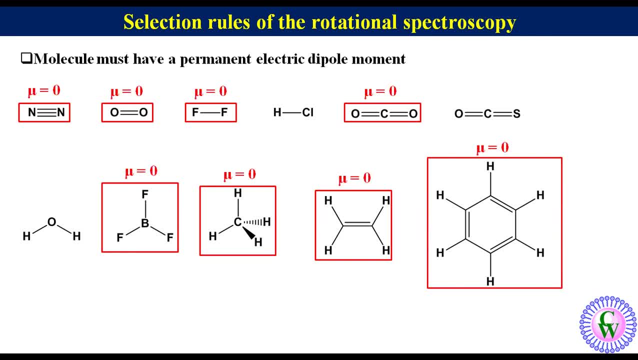 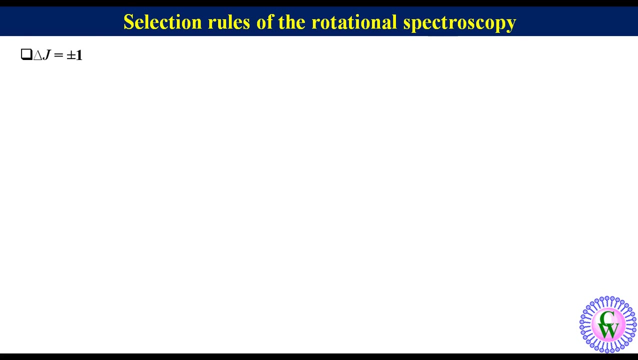 methane, ethylene and benzene have no permanent dipole moment, So these will be rotationally inactive, while HCl, carbon oxy, sulfide and water have permanent dipole moment and therefore these are rotationally active. Now let's discuss the second point, which is for allowed rotational transitions delta. 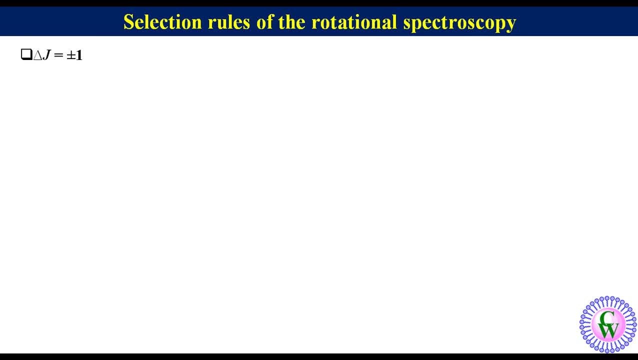 J is equal to plus minus 1.. This means only those transitions are allowed in which change in rotational quantum number is either plus 1 or minus 1.. Let's draw the rotational energy label of a rotationally active molecule: Delta J is equal to plus 1. means difference between the rotational quantum number of the 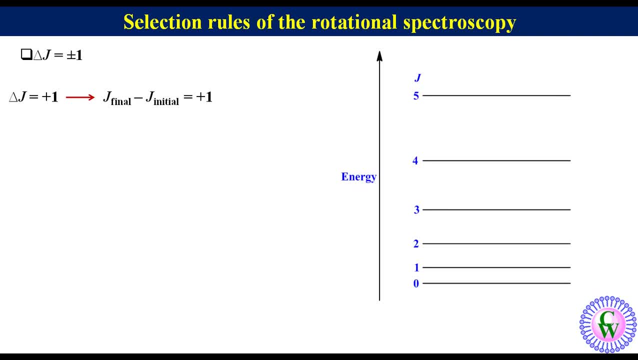 final label and the initial label is plus 1.. This corresponds to the absorption. These transitions will be from 0 to 1, 1 to 2, 2 to 3,, 3 to 4,, 4 to 5, etc. 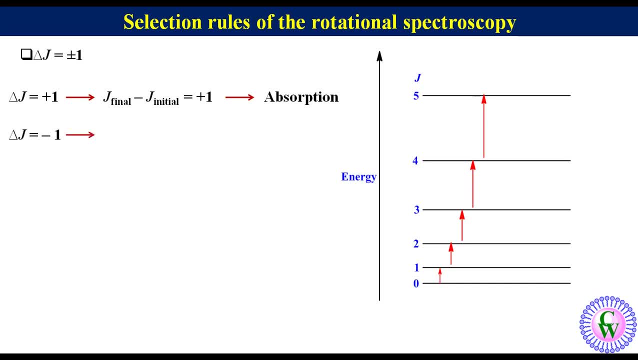 Delta J is equal to minus 1 means difference between the rotational quantum number of the final label and initial label is minus 1.. This corresponds to the emission. Delta J is equal to minus 1 means difference between the rotational quantum number of the final label and initial label is minus 1.. 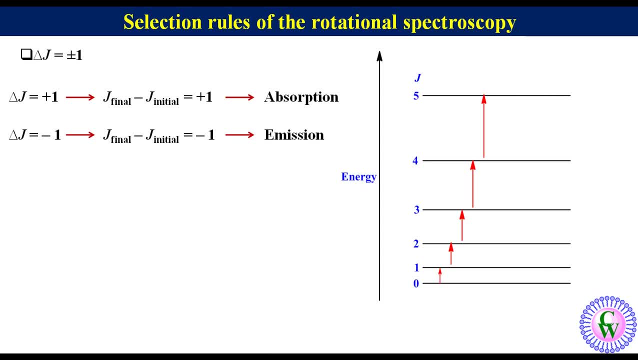 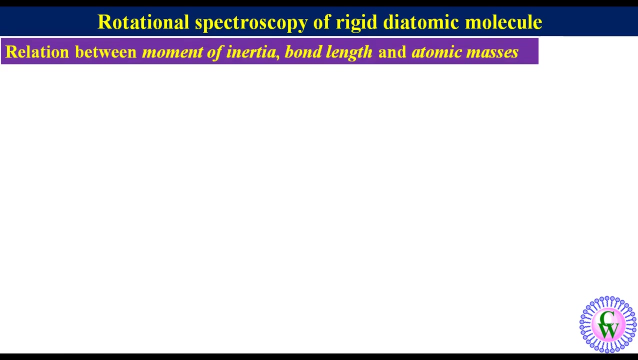 These transitions will be from 1 to 0,, 3 to 1,, 3 to 2,, 4 to 3,, 5 to 4, etc. Rotational spectroscopy of rigid diatomic molecules. In this we will first discuss relation between moment of inertia, bond length and atomic. 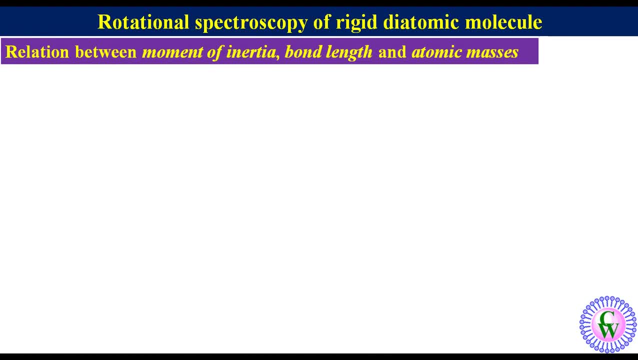 masses, Even though the diatomic molecules are not rigid. we are just supposing it to be rigid. Suppose we have a heteronuclear diatomic molecule with the mass of heavier atom M1 and lighter atom M2.. The center of mass of the molecule will lie towards the heavier atom, somewhere over here. 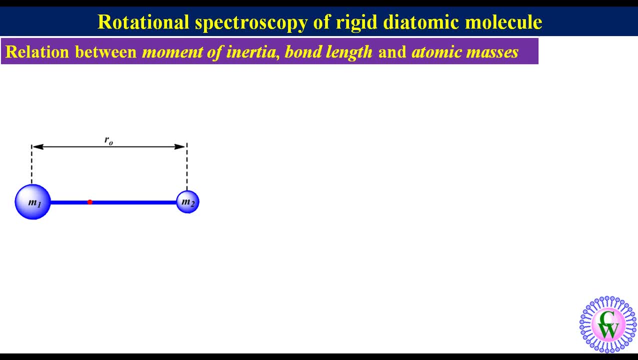 The bond length is 0.5.. The distance between the center of heavier atom and the center of mass of the molecule is R1.. The distance between the center of lighter atom and the center of mass of the molecule is R2.. These are the three mutually perpendicular axes A, B and C passing through the center. 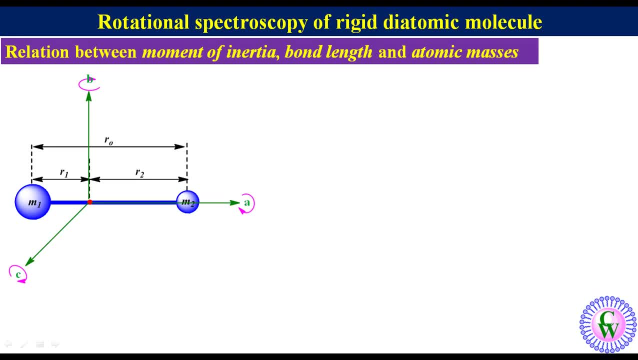 of mass of the molecule. The moment of inertia associated with these two diatomic molecules is known as the moment of inertia. These axes are Ia, Ib and Ic. Here Ia is equal to 0 and Ib is equal to Ic. 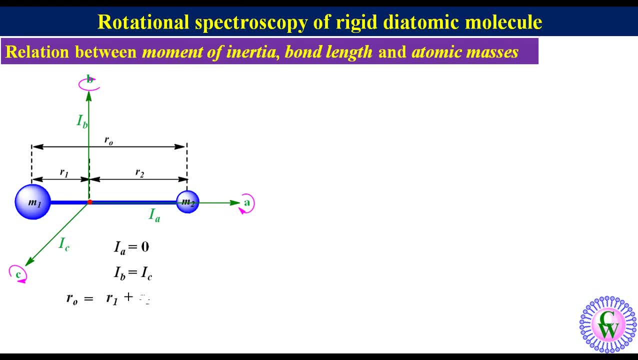 We can see that R0 is equal to R1 plus R2.. Label this as equation number 1.. M1, R1 is equal to M2, R2. label this as equation number 2.. We have seen that Ib is equal to Ic. 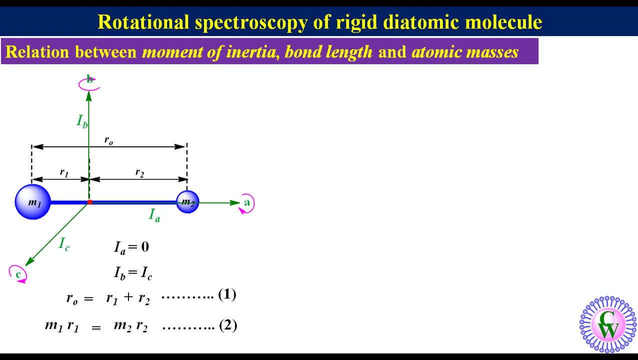 So we have seen that the moment of inertia is equal to Ic. So we have seen that the moment of inertia is equal to R1 plus R2.. We can choose any one of them for our discussion, but by convention Ib is taken under consideration. 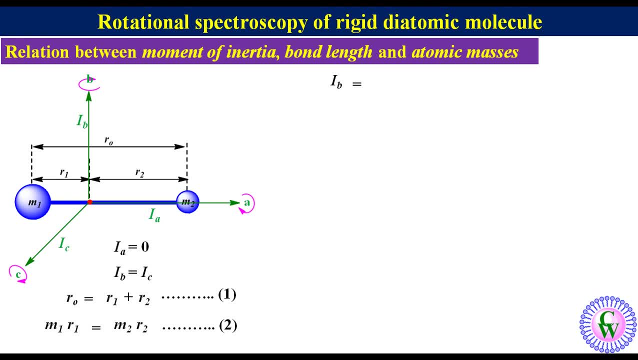 So we can write: Ib is equal to m1- R1 square plus m2 R2 square From equation number 2, we know that m1 R1 is equal to m2- R2.. So we can write: Ib is equal to m2- R2- R1 plus m1 R1- R2, or Ib is equal to R1- R2 into m1 plus. 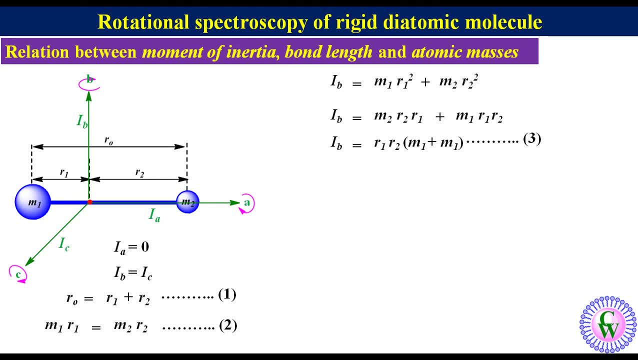 m2.. This is equation number 3.. We can write: m1 R1 is equal to m2 R0 minus R1 is equal to m2 R1 plus m2 R2.. So we can write: Ib is equal to m2 R2 plus m2 R2.. 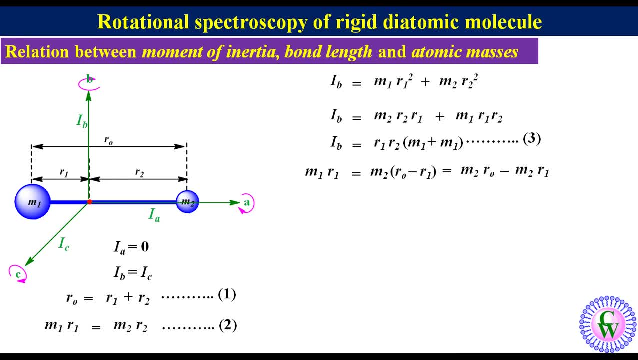 So we can write: m1 R1 is equal to m2 R0 minus m2 R1.. So R1 is equal to m2 R0 upon m1 plus m2.. And similarly we can write: R2 is equal to m1 R0 upon m1 plus m2.. 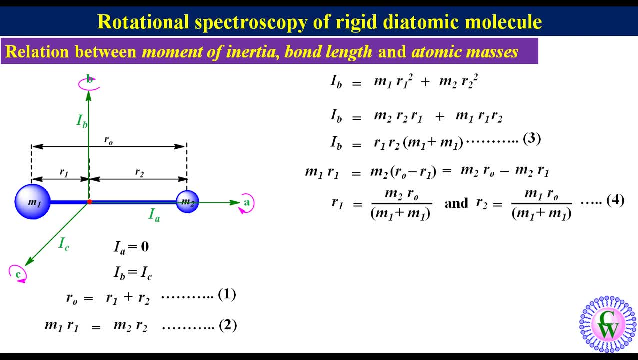 This is equation number 4.. Putting the value of R1 and R2 from equation number 3, equation number 4 into equation number 3, we will get. Ib is equal to m1 into m2 upon m1 plus m2 into R0 square. 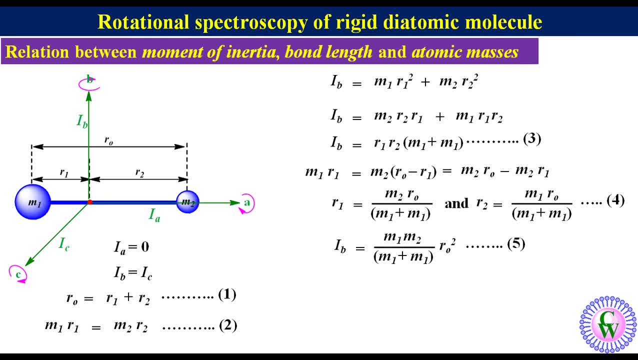 This is equation number 5.. m1 into m2 upon m1 plus m2 is called reduced mass And it is denoted by mu. So we can write: Ib is equal to m2 R0.. This is equation number 6.. 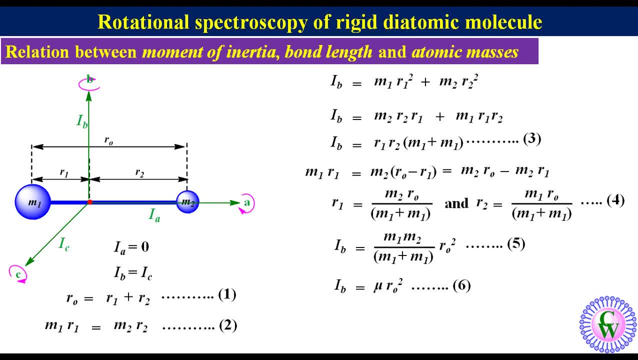 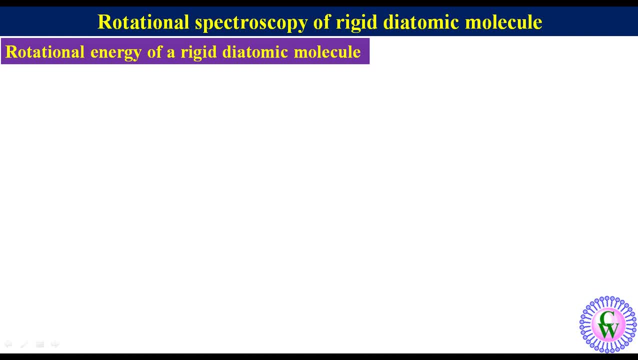 This equation shows the relation between moment of inertia, bond length and atomic masses. Rotational energy of a rigid diatomic molecule. Rotational energy of a rigid diatomic molecule in Jth rotational level is given by EJ- is equal to H square. 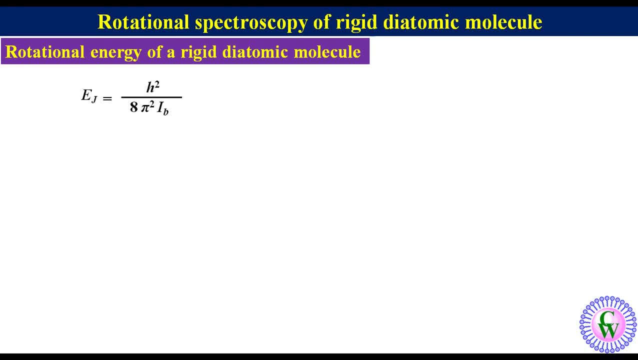 upon 8 pi. square i b into j, j plus 1 joules, where j is equal to 0,, 1,, 2,, 3, etc. and h is Planck's constant. Dividing both the sides of this equation by h? c, we will get e j upon h c. 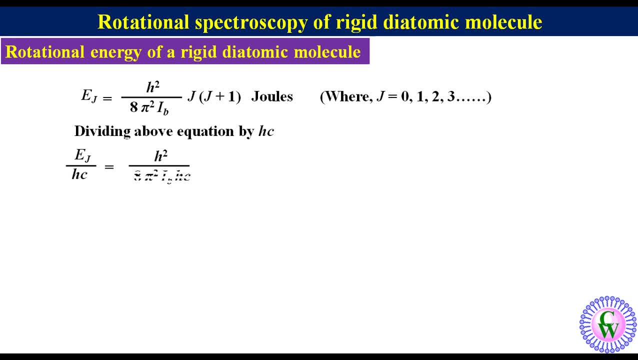 is equal to h square upon 8 pi, square i, b into h, c, into j, j plus 1 centimeter inverse, where c is the velocity of light in centimeter. second inverse. This is the wave number. So we can write: wave number is equal to h upon 8 pi square i b into c, into j, j plus 1,. 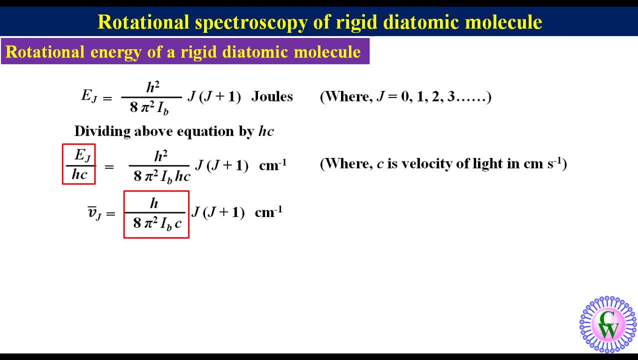 centimeter inverse. This part is called rotational constant and is denoted by capital B. So we can write: wave number is equal to capital B, j, j plus 1 centimeter inverse, where b is equal to h upon 8 pi. square i, b into c. Rotational energy levels of rigid diatomic molecules. 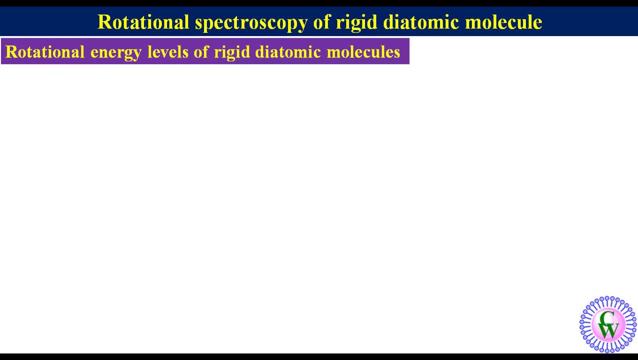 we have seen that wave number associated with a particular rotational level, j is equal to b, j j plus 1 centimeter inverse where j is equal to 0, 1, 2, 3, etc. So wave number for j is equal to 0. that is, ground state label is equal to b into 0, into 0 plus 1 is equal to 0.. 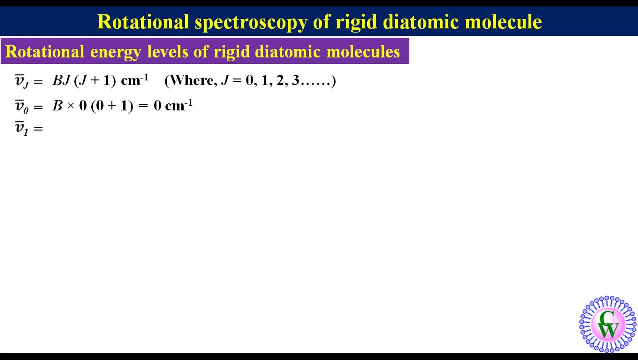 Wave number for j is equal to 1 is equal to b into 1. into 1 plus 1 is equal to 2b. centimeter inverse For j is equal to 2, it will be equal to b into 2. into 2 plus 2 is equal to. 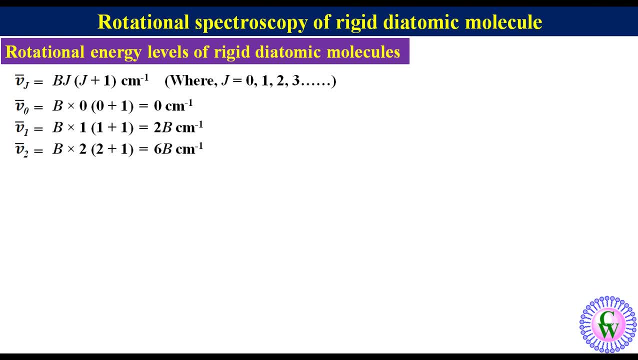 6b centimeter inverse. inverse. For j is equal to 3, it will be b into 3 into 3 plus 1 is equal to 12 b centimeter inverse. Similarly, for j is equal to 4 and j is equal to 5, wave. 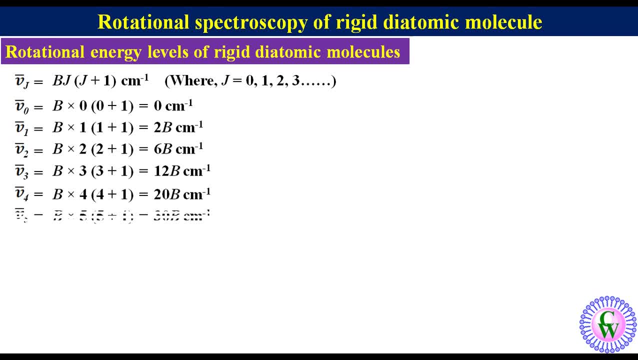 numbers will be 20 b and 30 b. centimeter inverse Difference between the wave number of two adjacent energy levels will be equal to wave number of j plus 1 level minus wave number of the jth level. That will be equal to b j plus 1 j plus. 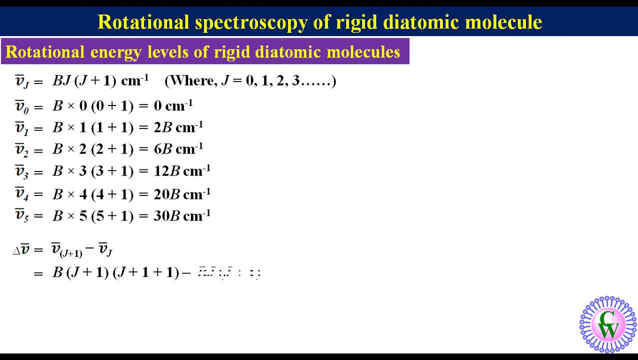 1 plus 1. minus b j into j plus 1 is equal to b? j plus 1. into j plus 2. minus b j j plus 1 is equal to b? j square plus 2 j plus j plus 2. minus j. square minus j is equal to 2 b j plus 1.. So from this equation we can calculate: 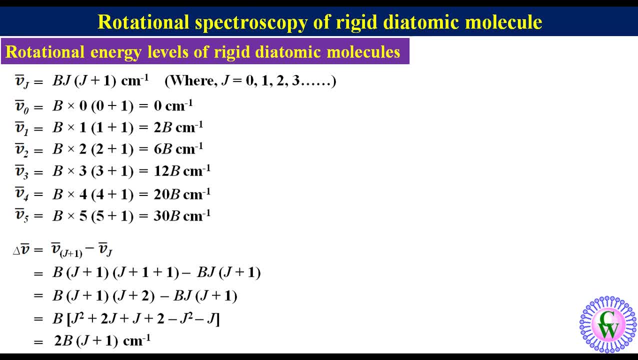 energy difference or wave number difference between two adjacent rotational levels. Thus we can show different rotational levels like this: These are the 1st, 2nd, 3rd, 4th and 5th absorption rotational transitions, The wave number corresponding to a particular 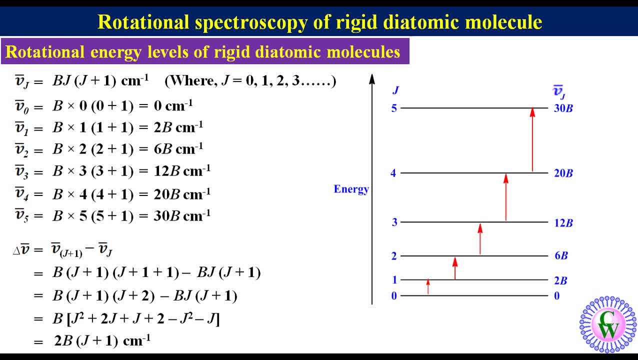 transition is equal to the difference between the wave number of the two levels. So the wave number for the 1st, 2nd, 3rd, 4th and 5th transitions will be 2b, 4b, 6b, 8b and. 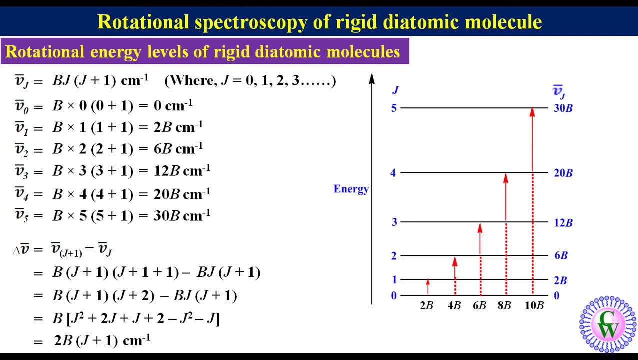 10b. Here we can see that the separation between two adjacent rotational lines is equal to 2b centimeter inverse. Thus we can find the value of b for the first, 2nd, 3rd, 4th and 5th transitions. This is: 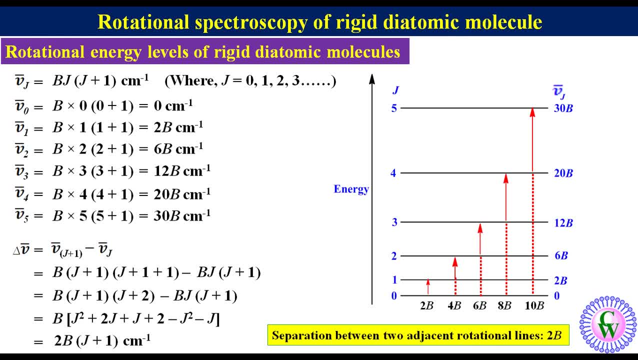 equal to 2b centimeter inverse. Thus we can find the value of b for the second, 3rd, 4th and 5th transitions. Now we can see the value of b from the rotational spectrum just by separation between two adjacent 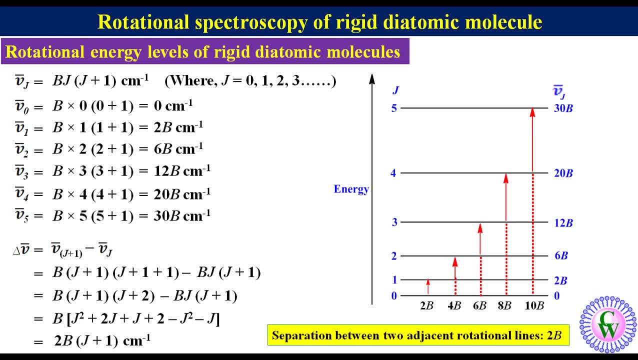 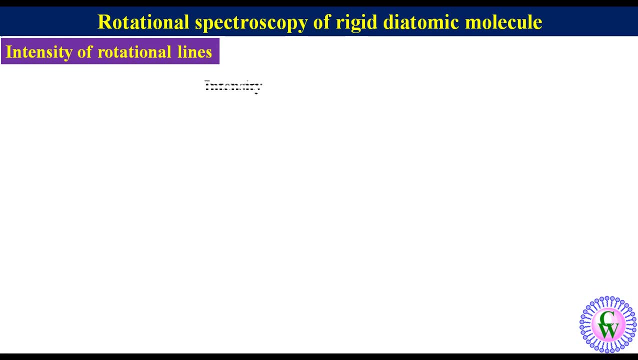 lines. Once we know the value of b, we can find moment of inertia and bond length of the molecule. Intensity of the Rotational lines. The intensity of a rotational line for the rotational transition from the jth rotational level is equal to the internal force of the element In this.